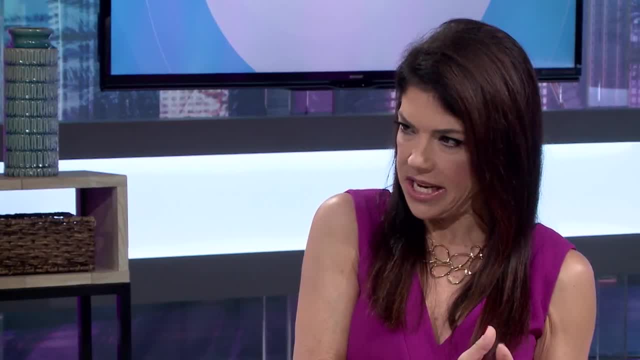 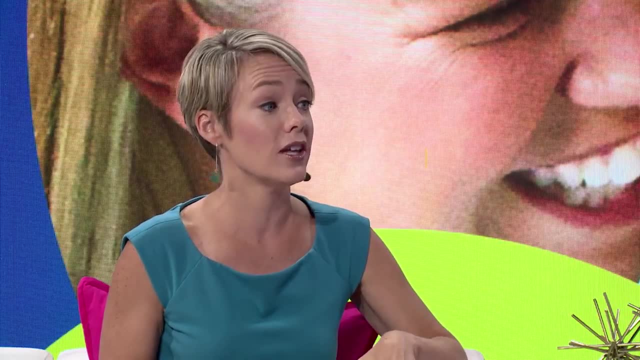 Balance and your program not only just helps children with ADHD, it goes beyond that with other diagnosis right, Absolutely. in fact, probably about half of the children in our centers don't have a label or diagnoses at all, but they simply struggle. so a lot of the kids 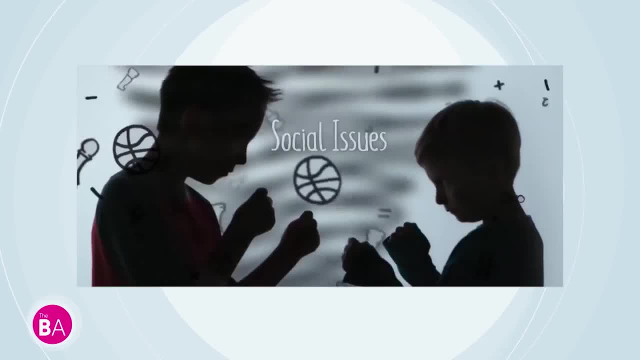 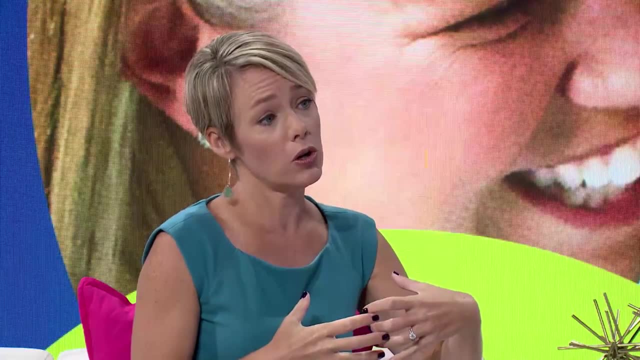 that we work with may struggle with paying attention in class, getting their homework done and turned in. they may struggle making and keeping friends. they may struggle keeping up academically. so the kids that we work with have areas of struggle that we're able to have a 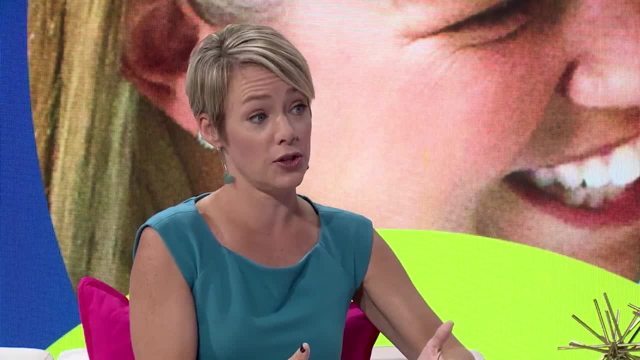 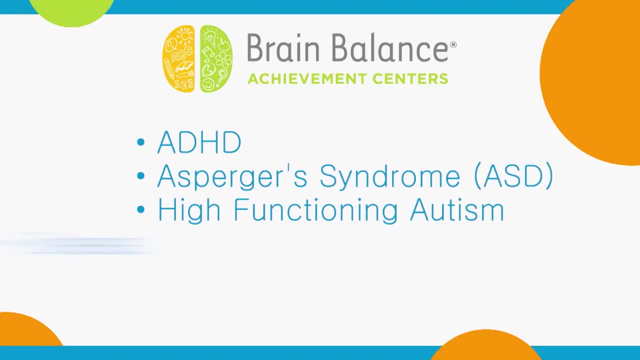 positive impact on and change. now many kids in center do also have labels. so we work with a lot of children with labels such as ADHD, Asperger's, high-functioning autism, different learning disabilities, dyslexia. the list sort of goes on and on. but that common denominator is: we work. 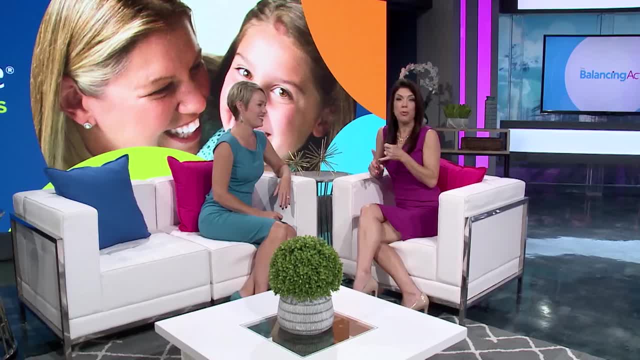 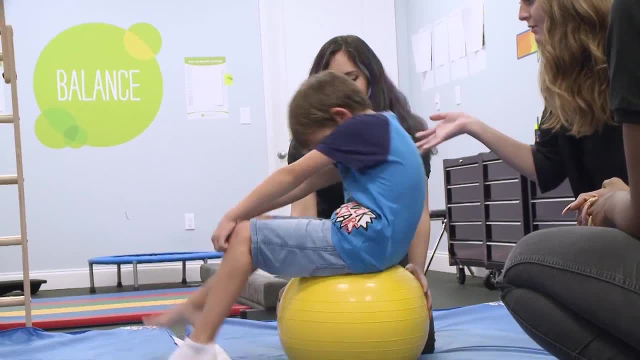 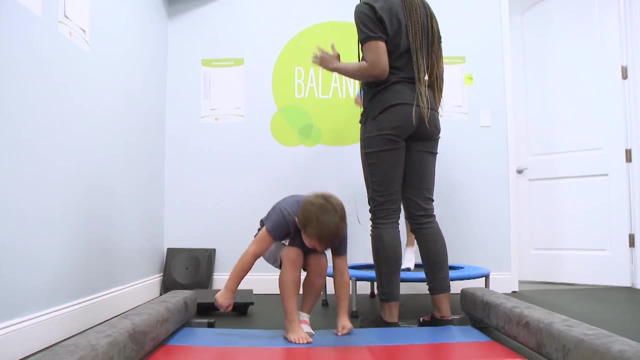 with kids that struggle and we're able to help make things better. We went to the Brain Balance Achievement Center in Pembroke Pines, Florida. it was really great to be there. take a look. Four, five, Bring your knee up a little bit higher. 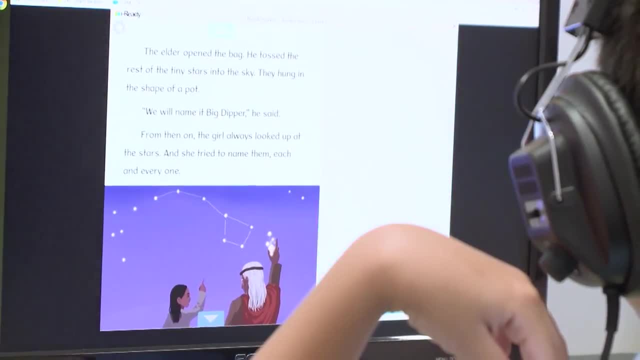 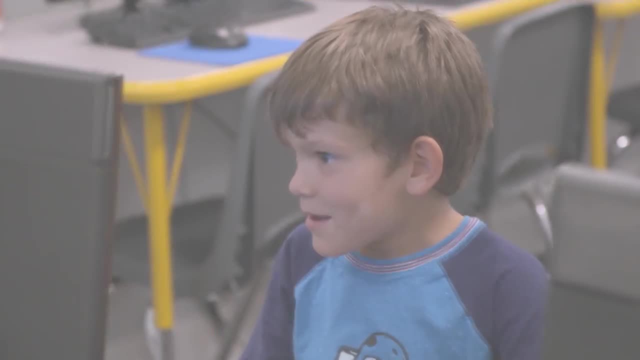 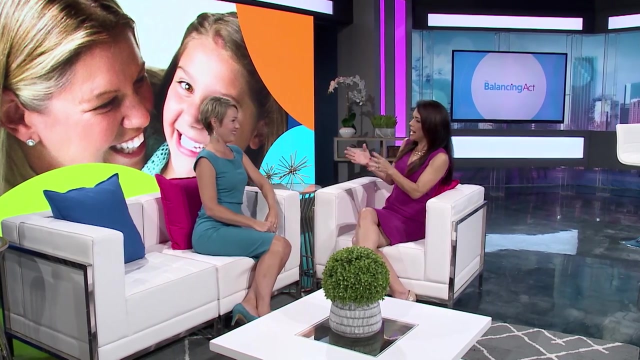 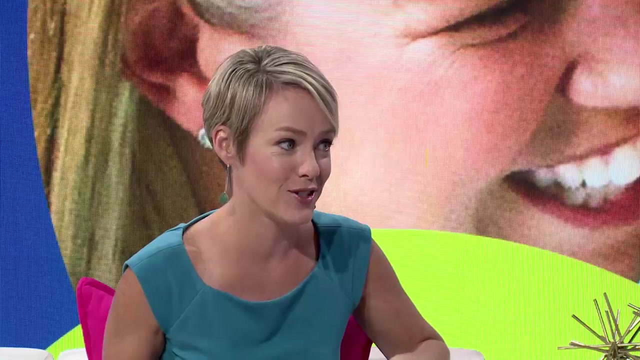 That's all, but it's going to bounce away. That was so great and a lot of fun. yes, all right. so how does it work? We all know that exercise is good for the body, but did you know that exercise is good for the brain? Common sense, right? So? 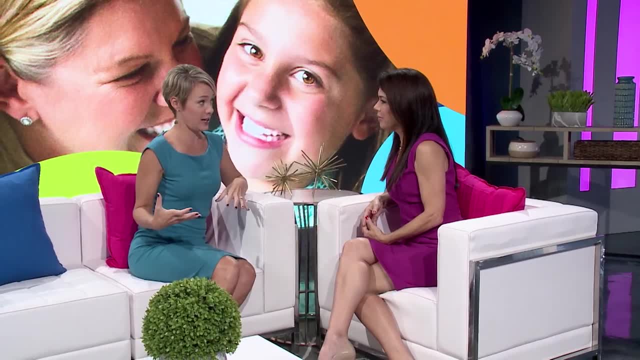 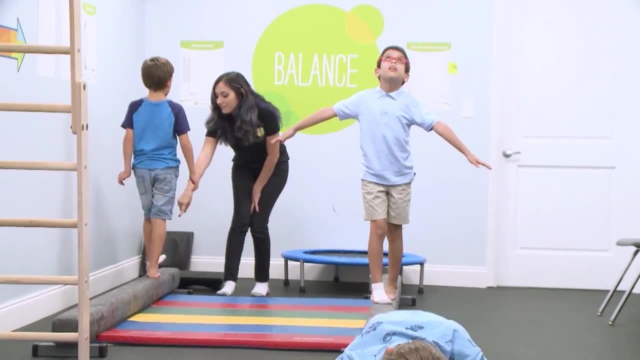 we're able to do very specific exercises and activities that wake up different parts of the brain. so when we start to utilize all of the different senses in our body in a very particular way, as well as physical activities involving coordination and timing, and not only do we do them- 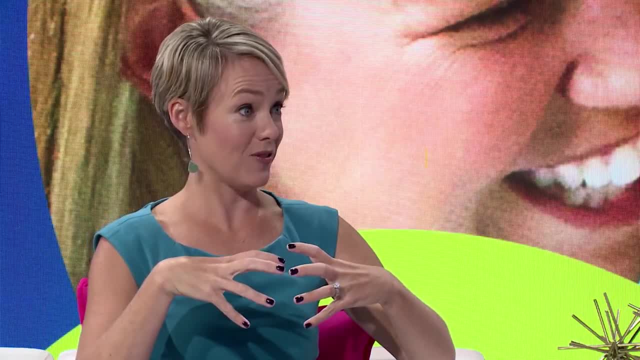 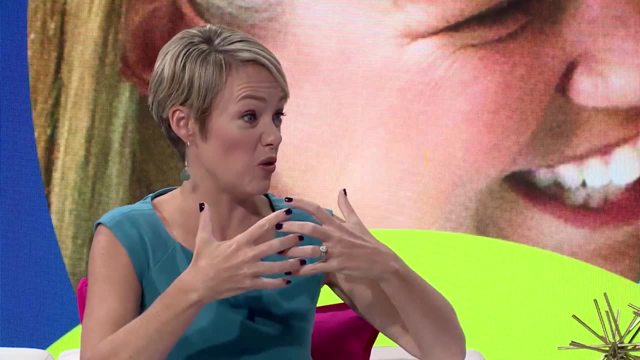 but we do them all at the same time to combine the effects. When we do this, it starts to wake up all these different regions of the brain and this starts to help to make things click and improve and we start to see better, more efficient function. Both of my children- 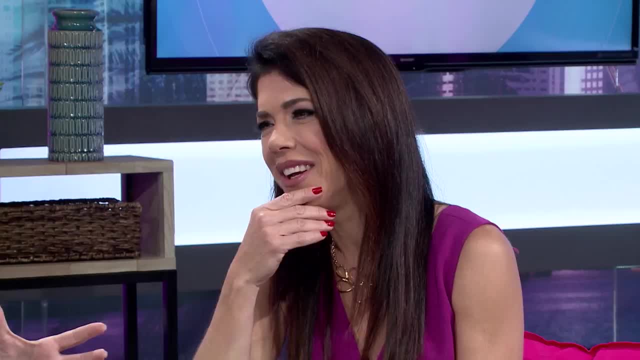 have gotten to do the program and my husband and I do this together, so this is sort of a family thing for us. in fact, if you go to the website, on the home page of the website and there's a couple of videos and I talked a little bit- 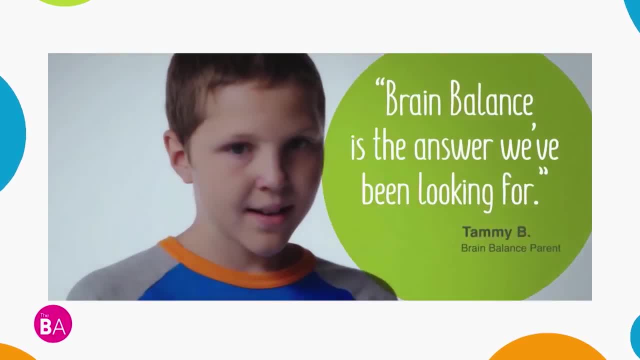 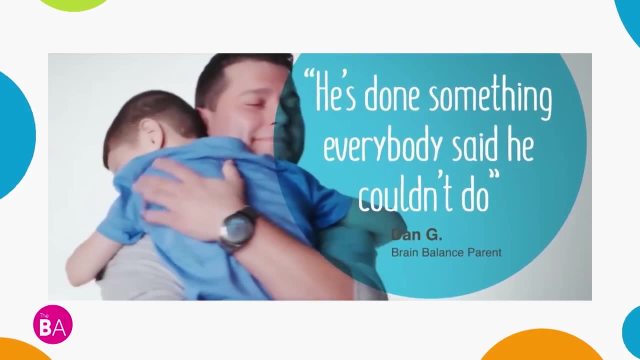 about my children and their experience on those videos. but beyond just being able to help our own children, we've gotten to work with family, with friends, with neighbors. we feel like we've really gotten to have an impact on our community. I even got to see it as 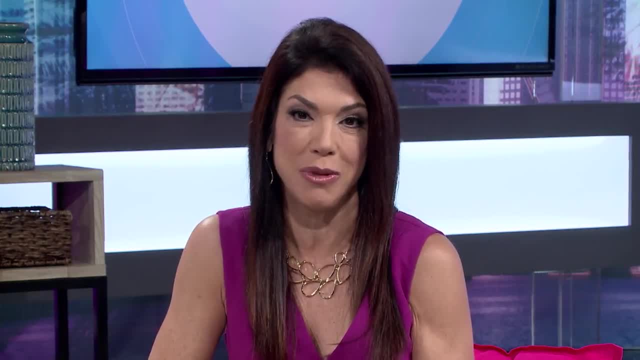 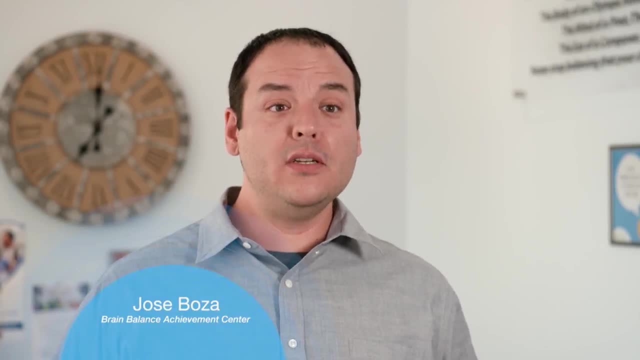 well, I got to sit down with two parents whose children go to the brain balance achievement center in Pembroke Pines, Florida, and here's what they had to say: very special In school. very similar he would want to do well, but then he would come home very distraught because he. 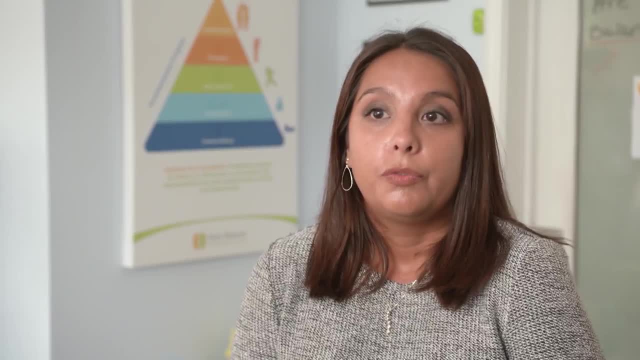 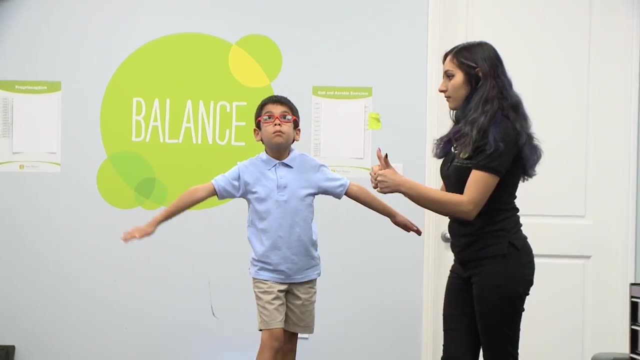 couldn't perform well or he thought he wasn't doing well. We look for resources to find the right teacher, to find the right treatment. We're looking for a mentor to find the right place, the right center. and when we came to brain balance, they opened our arms and said we 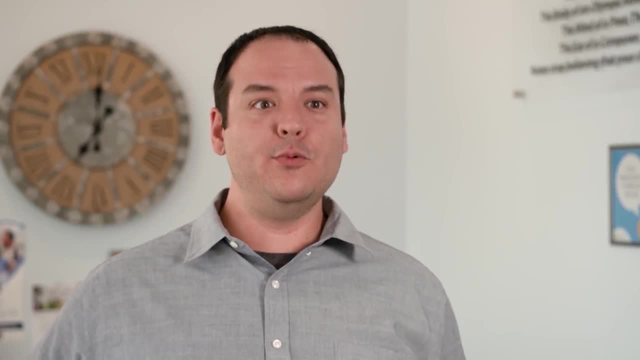 can help you. And now it's like, after bringing him to brain balance, it's like he's, he's with it, he's on the program, he gets it like he's just like up to speed on everything. it's like you wouldn't pick him out of the crowd like any. 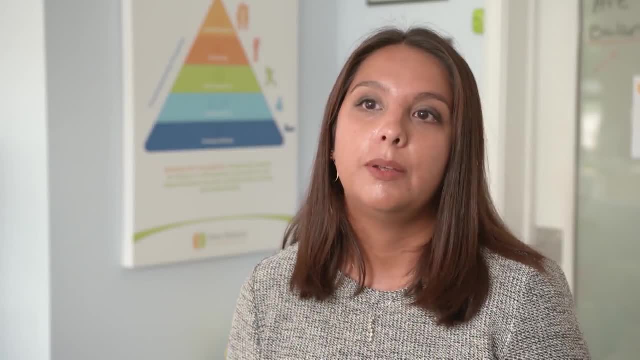 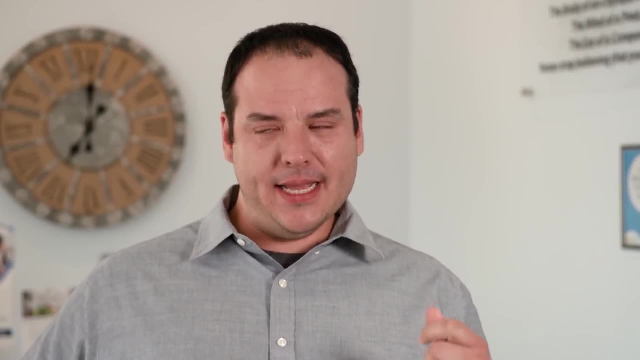 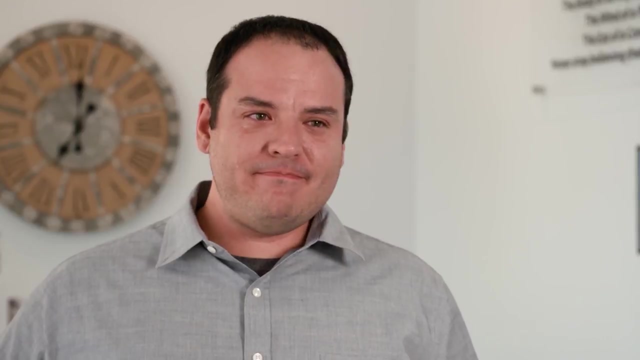 different from anybody else. Today my son will succeed, today my son will make it, And to see them struggle, sorry. and then you know, just to kind of turn it around, it's, it's fantastic, There's no other way to say it. it's a. 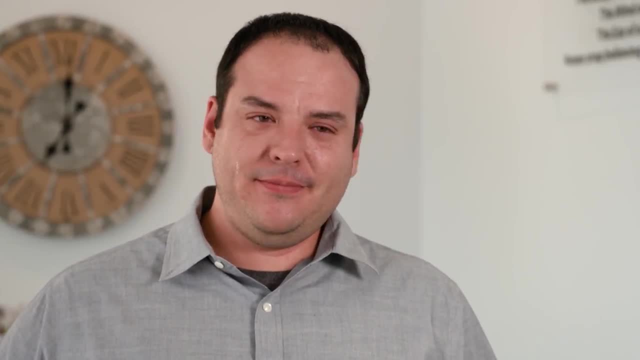 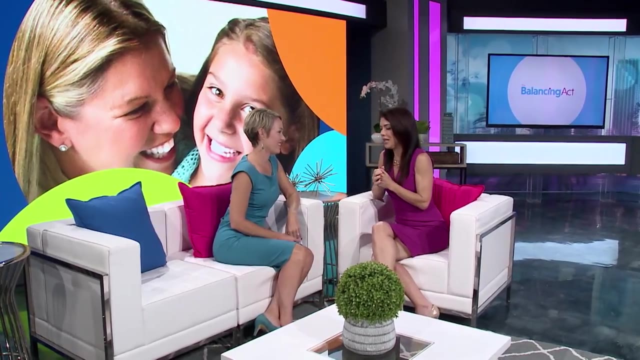 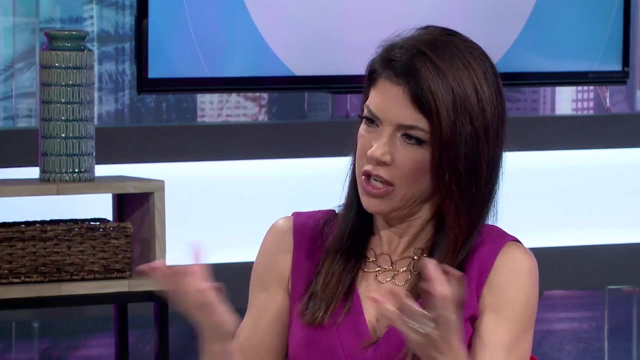 wonderful thing. How grateful are you? Super grateful? Why? Because I have my boy. It's just so great to hear a parent so happy because they want their children to succeed. it's just fabulous. Nationwide these centers are they? nationwide We are. we have over a hundred centers. 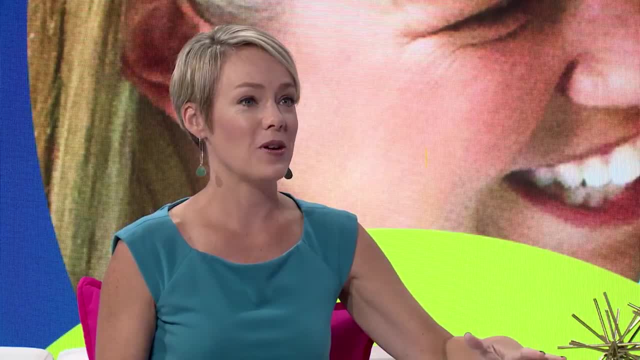 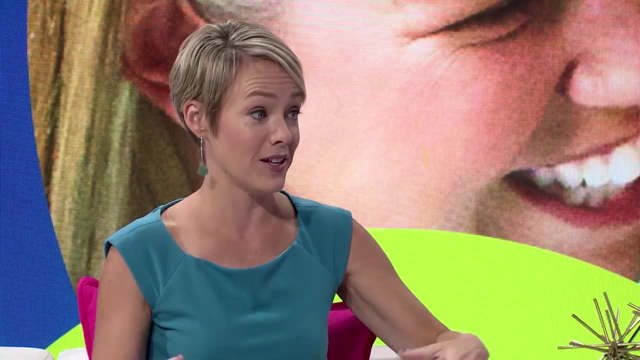 nationwide and so we get to help kids all across the country. But what's been so again neat and amazing to me is how many families we've had reach out to us beyond just the US. Just in my centers alone, we've had families come to us from New Zealand, from Australia. 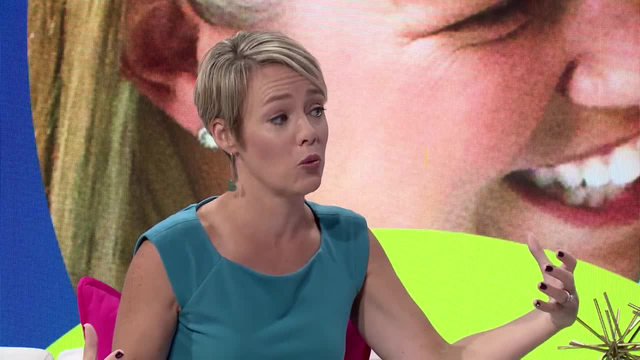 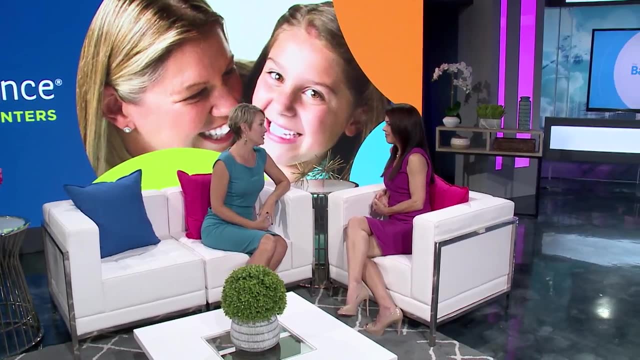 Wow, Other centers. we've had families from Turkey, from India, from all over the world. It's kids' struggle and we have an opportunity to reduce that struggle and make things better And as a parent, we do what we can to just set our kids up for success, like you said. 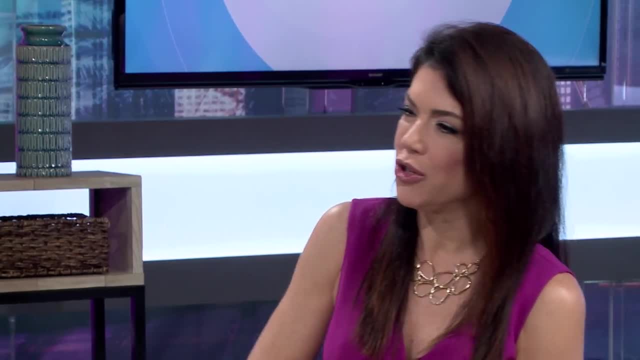 You're really making a difference. Thank you For our viewers who'd like more information on the Brain Balance Achievement Centers. where do they go? Brainbalancecom, Thank you. Thank you so much for being here and thank you for letting us go to the one in Pembroke.